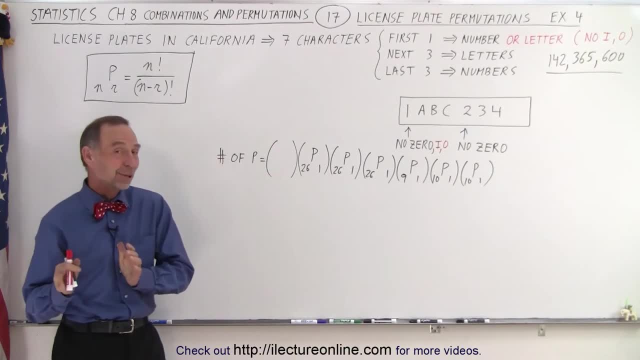 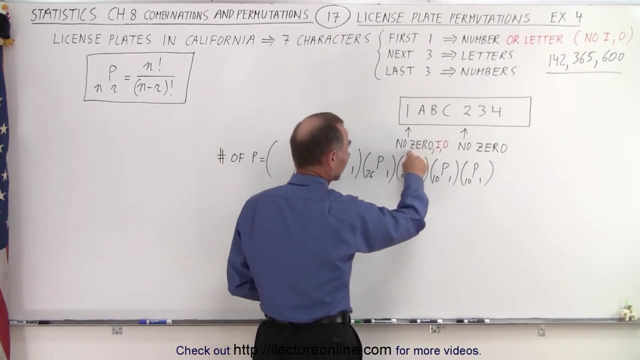 Welcome to Elector Online. As we mentioned in the previous video, in California we simply ran out of combinations- or actually, more properly said, permutations- on our license plates, Because we had seven characters. the first character had to be a number, but not a zero was allowed. 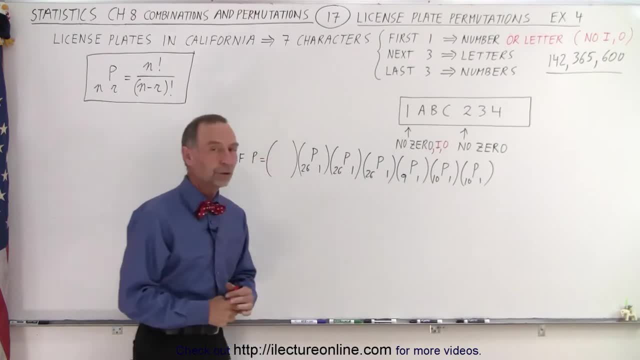 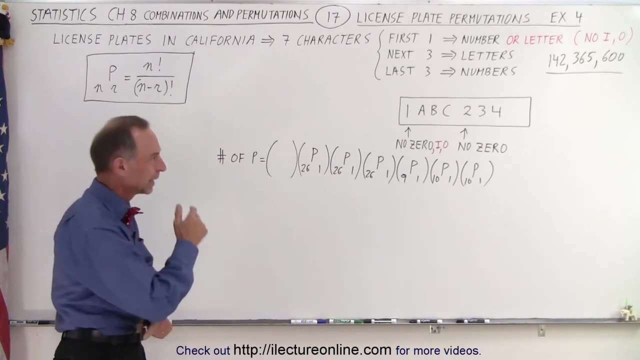 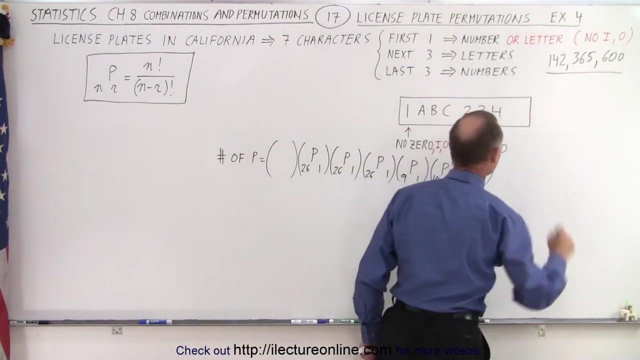 The next three were letters and then the last three were numbers, again and again, the first one was not allowed to be a zero, so they wouldn't confuse it as an O, for example. Now we ran out of combinations, or again permutations, even though we had over 140 million of them, so we decided to let the first character also be a letter. 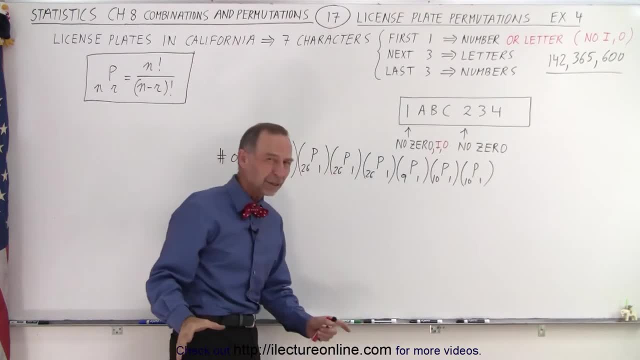 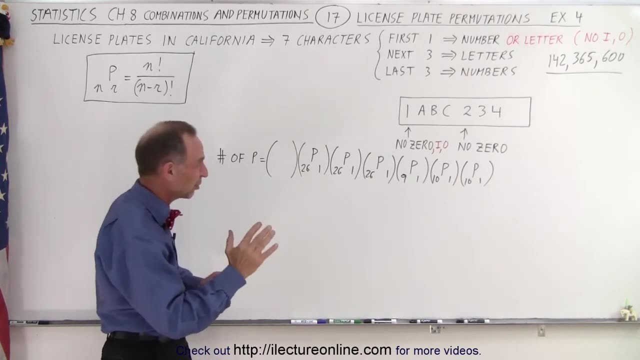 But it would make sense that an I or an O would not be allowed, because that would be too confusing with a one or a zero. Well, a zero wasn't allowed anyway, so we just don't want an O or a zero there, so it makes more sense. 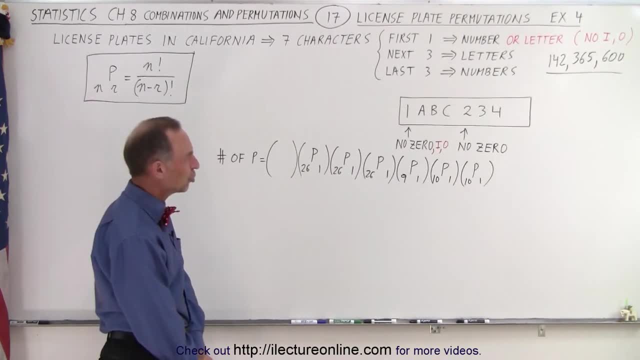 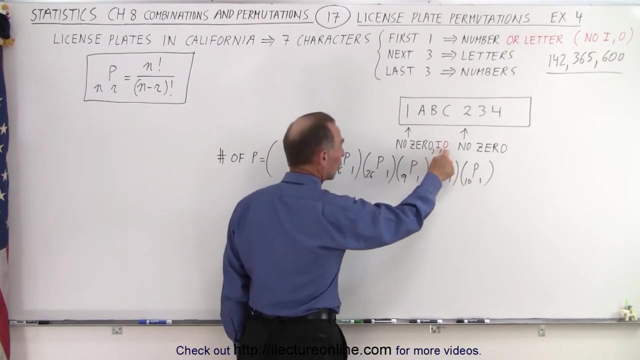 Now, how do we make? How do we make that change? Well, the only thing that has to change is the number of permutations for the very first character. So it could be a letter or a number. There's 26 letters, 10 numbers, that would be 36, but a zero was not allowed, an I is not allowed and an O is not allowed. 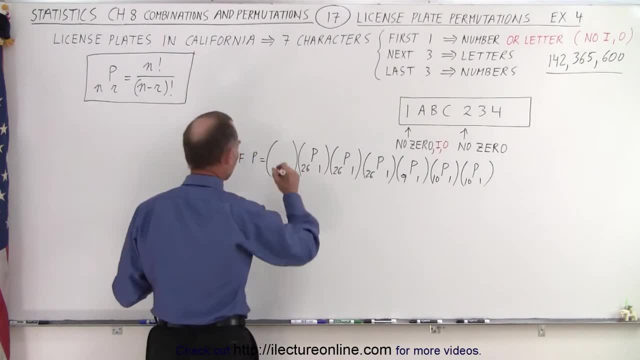 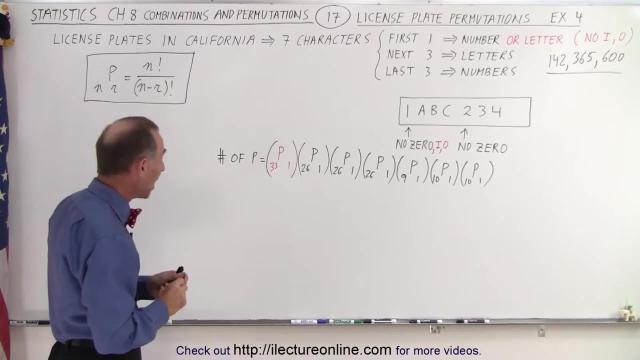 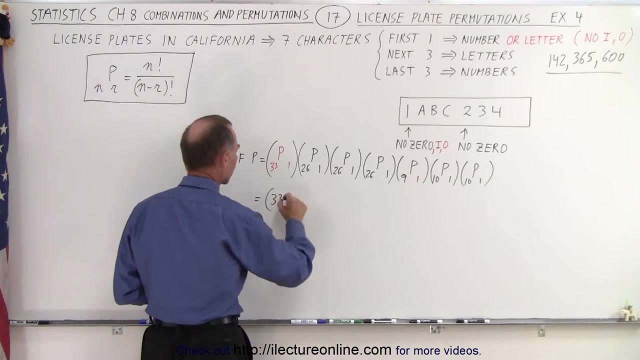 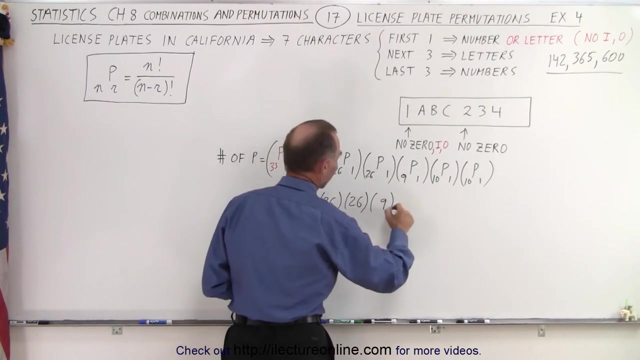 So we subtract three from the 36, that gives us 33.. So now we have P331, and now we have to calculate the new amount of permutations. So in this case this is equal to Well, that would be 33 times 26,, times 26,, times 26,, times 9,, times 10, and times 10.. 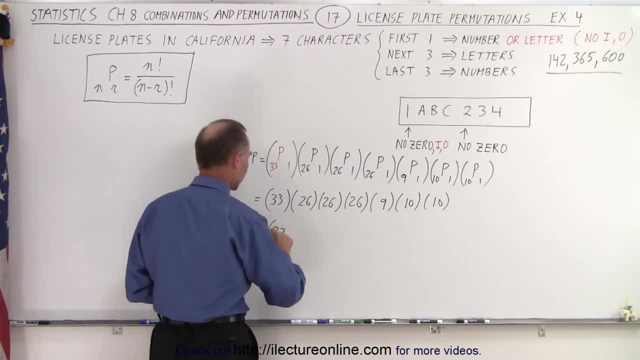 Of course we can write that in a more compact form: 33 times 26 cubed, times 9, times 10 squared, So let's see how many total permutations we have this time. So we have 33 times 26 cubed. 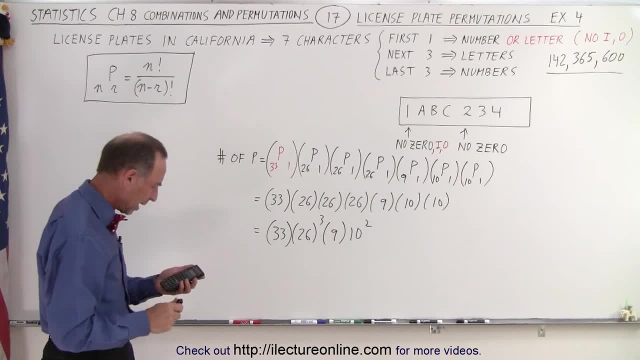 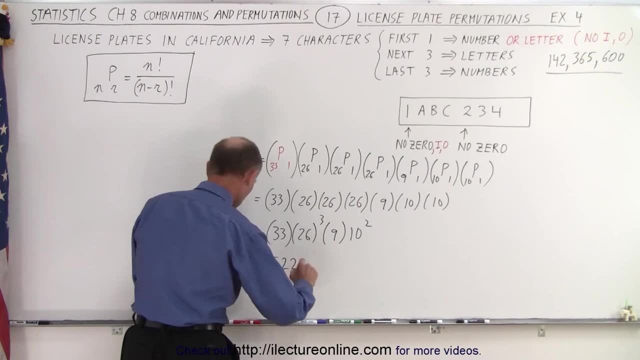 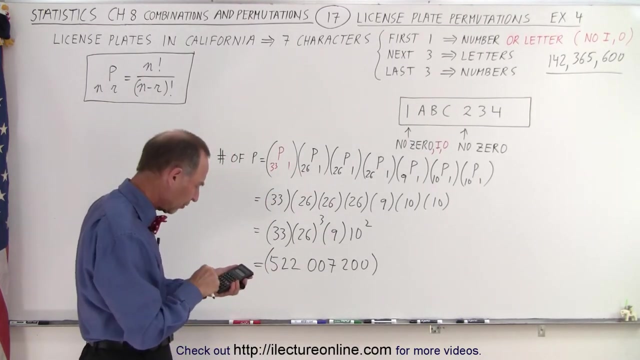 Times 9, times 100, and that now gives us, wow, quite a few more. Now we have as many as 522,007,200.. Now, if we subtract from that the ones we already had because we can't reuse those, so minus 142,365,600,. 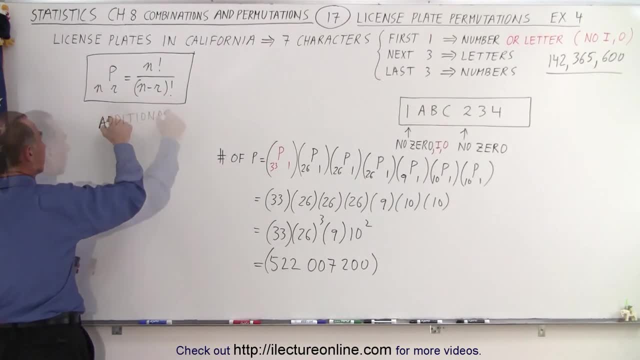 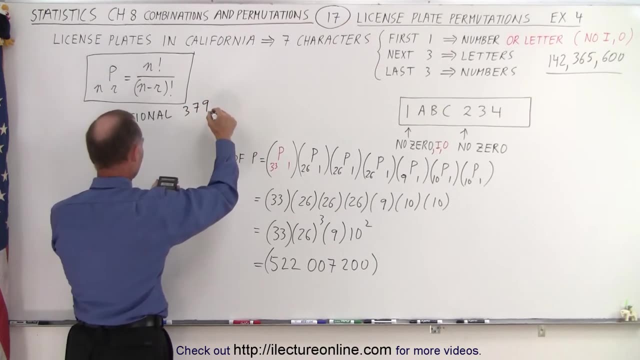 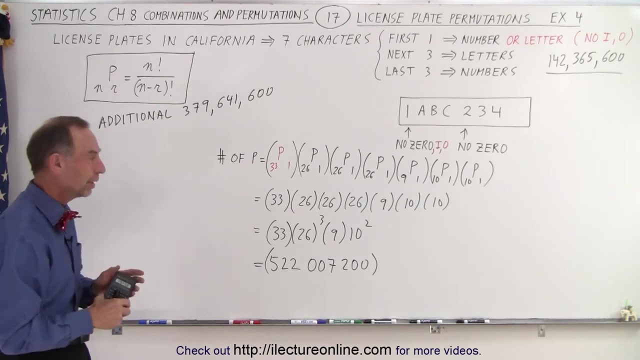 that leaves us with an additional 379,641,600.. And notice, essentially, when you look at that number, look at this number, we've almost added another three times as many, about two and a half times as many numbers as we had before. So that should probably last us for another 30 or 40 years in California until they have to make another change. maybe more letters in the back instead of numbers. Maybe we'll make the last character a number. that would add another whole bunch of permutations. 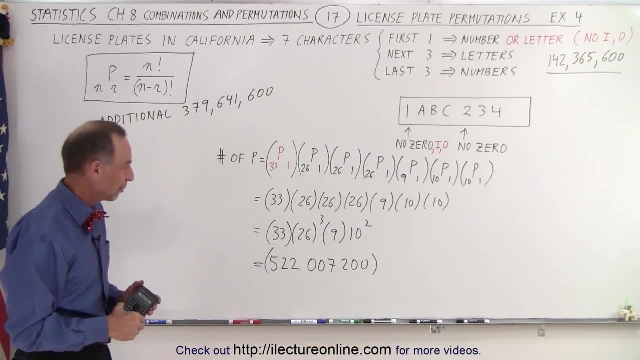 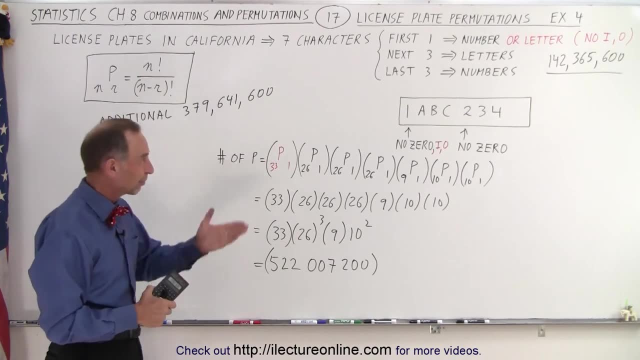 or maybe we'll go to an eighth character. We'll see what happens when we get that far. But at least notice we went from 142,000,000 to 522,000,000.. So that's a big plus by making that one little change in the front instead of just a number. 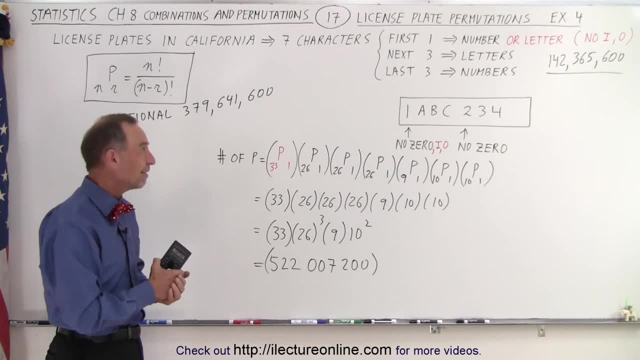 without having a zero as a possibility, We can add 24,000,000.. Or more letters, because we're not allowing I or an O, And that is how it's done, So we're good for now. 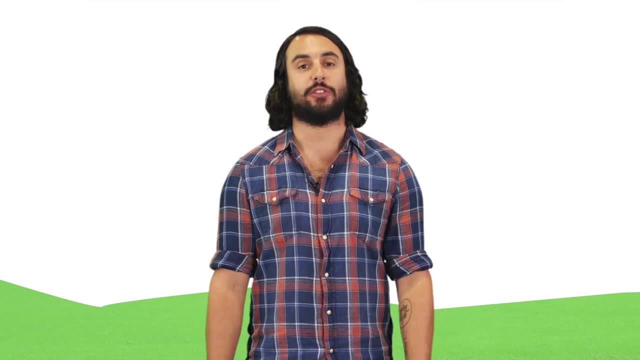 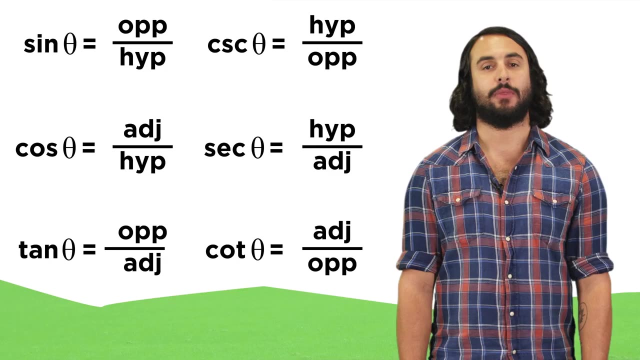 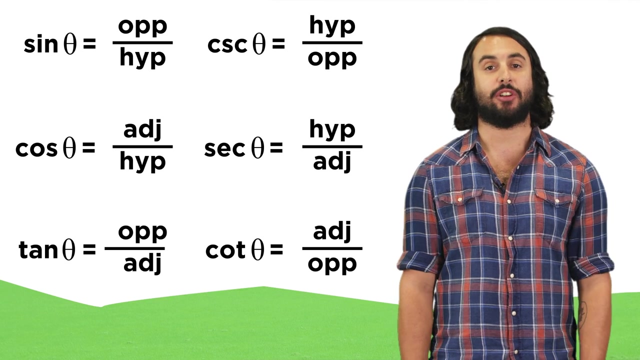 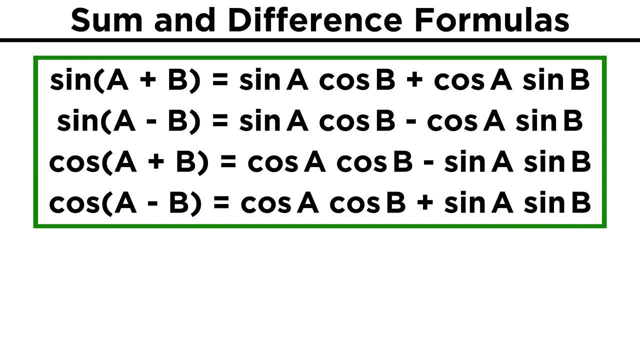 Professor Dave, here let's learn some important formulas for trig functions. I know that you've probably had enough of trig functions for a while, but there are some important formulas to mention, so let's knock them all out in one clip. First, the sum and difference formulas for sine and cosine, which are as follows: 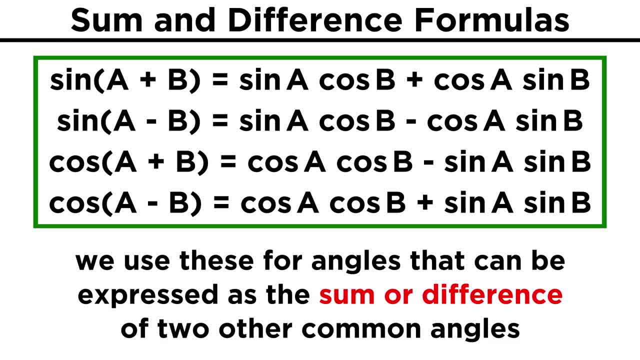 These tell us that if we want to find the sine or cosine of an angle, that is, the sum or difference of two other angles, we can find it in terms of the sine and cosine of those two angles. There are derivations for these but they are a bit involved so we won't go over.